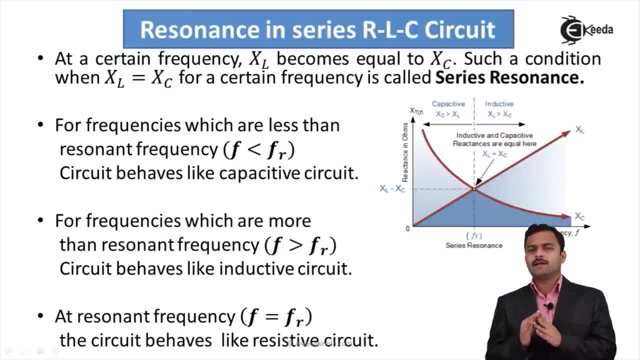 And inductor will act as a redundant, leaving behind only resistive circuit. So at certain frequency x l becomes equal to x c. such condition is called as series resonance. So what happens before series resonance and what happens after series resonance? Let us check it For frequencies. 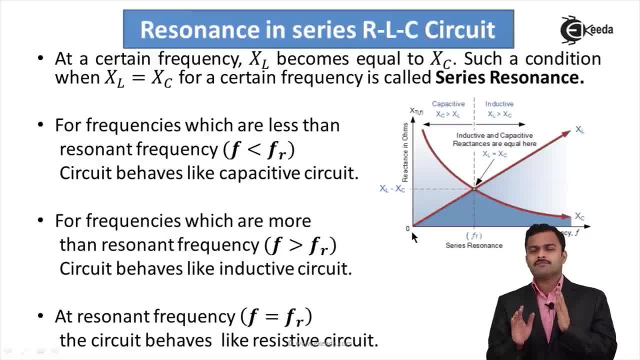 which are less than resonating frequency. resonating frequency is nothing but that frequency where resonance occurs. So before resonating frequency, if you check the graph, x c have higher values compared to x- l. So capacitive nature of circuit will be illustrated Now. 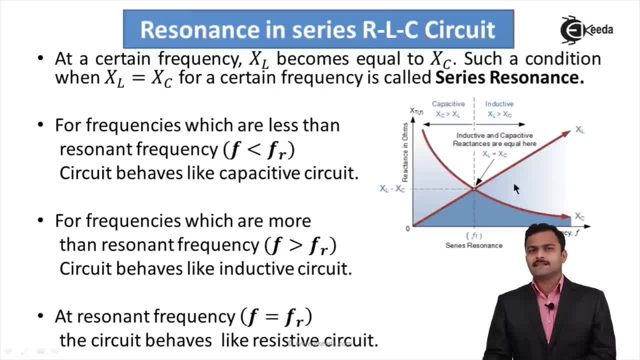 beyond resonating frequency I can say x, l is greater than x c. Circuit behaves like inductive circuit because L is dominating factor over c. But what happens at resonating frequency? So when both x l and x c is equal, circuit will be resistive in nature. Now this is 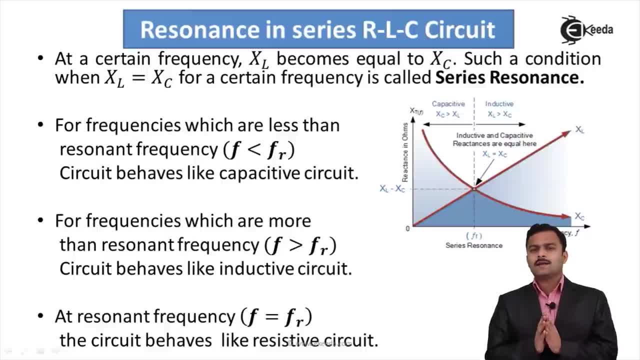 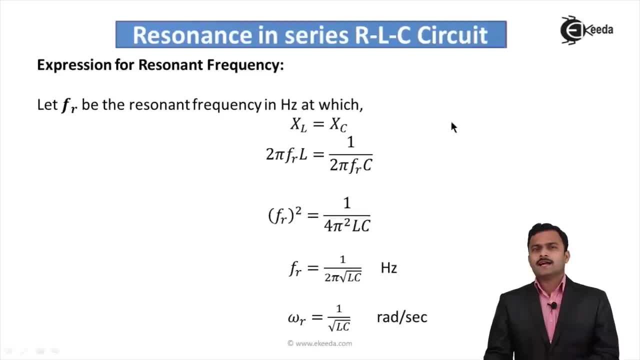 all about the phenomenon called series resonance. Now, what are the effects on circuit because of this resonance? we will see in the next slide. Before that, let us derive the expression for resonating frequency. So let f? R be the resonating frequency in Hertz, at which x? l. 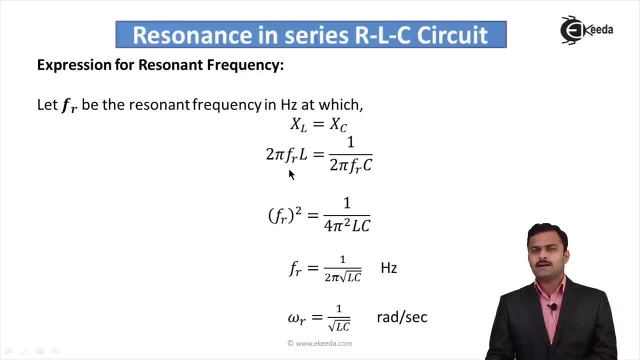 becomes equal to x c, 2 pi F R L. that is equal to 1 upon 2 pi F R C. If I solve, I will get F R square equal to 1 upon 4 pi square L C and taking a root I will get F R as 1 upon 2 pi root of L into. 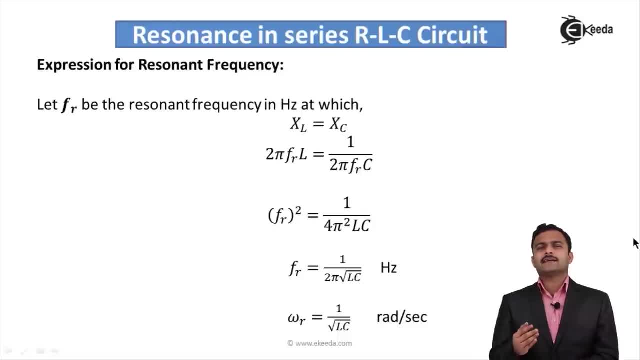 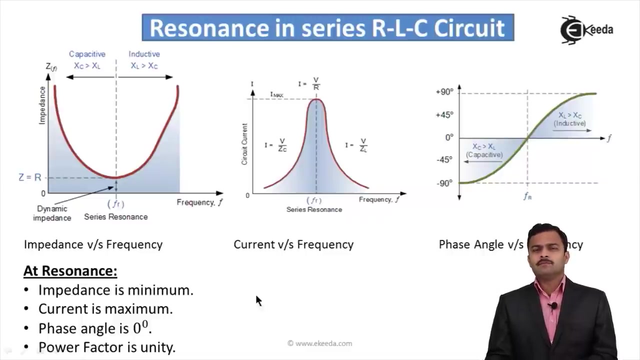 C hertz. Same frequency I can write in terms of radian per second. So that is equal to omega R 1 upon root of L C radian per second. What happens when resonance occurs? Let us see Next slide Lowerslide. So what happens at resonance? impedance becomes minimum Before. 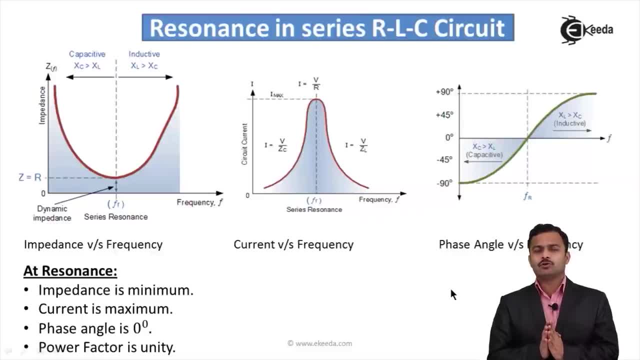 resonance. after resonance, impedance is given using root of R square plus X, L minus X C whole square. At resonance xl becomes equal to xc. So impedance will become equal to resistance of a circuit only, and that will be a minimum value. So the nature of impedance versus frequency will. 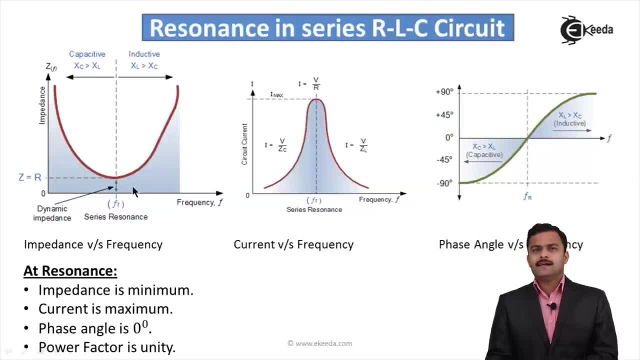 be like this In this region as well as in this region. impedance is more, but only at resonance. it is minimum, and that is equal to R. Secondly, current in a series circuit current is given by V upon Z. Whenever I say impedance is minimum, at resonance obviously. 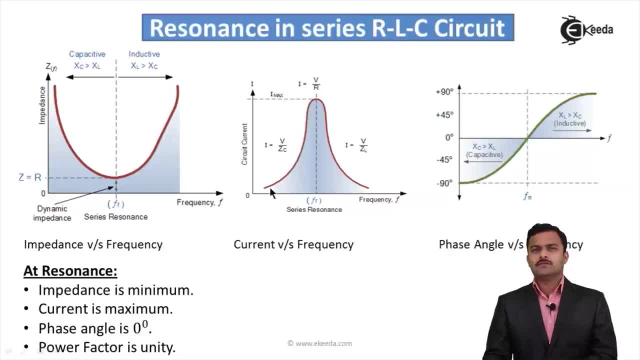 current will be maximum. So the nature of current versus frequency will be like this: Only at resonance current will have maximum value and that is given by V divided by Z, minimum, which is equal to R. So V by R will be the maximum current at resonance Phase. 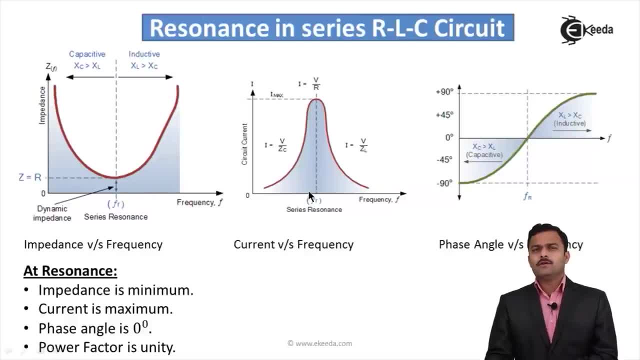 angle From the waveform or characteristic it is clear before. resonance circuit will be capacitive in nature, So for capacitance the angle will be negative. that we have discussed earlier. At resonance circuit will be resistive. angle will be zero. I am talking about a phase angle. 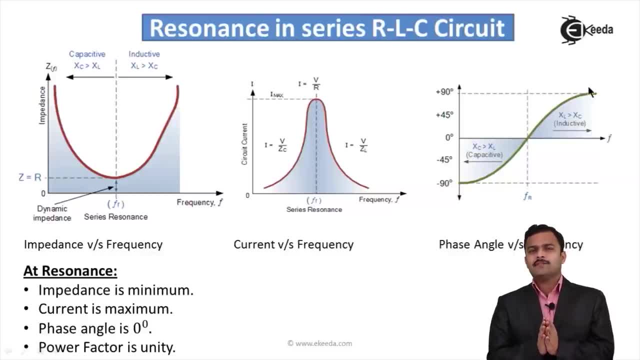 and beyond. resonance circuit will be inductive. angle for inductive circuit is positive. So the phase angle versus frequency will be like this: If I take a cosine of that, what I will get- cosine of zero degree- is one which is the maximum value of cos phi. So what happened at resonance power factor? cos phi is maximum. 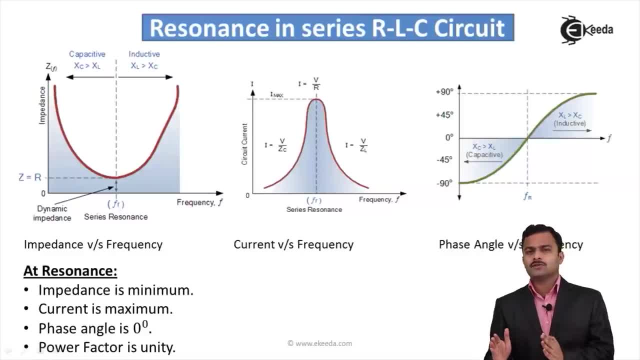 and that is equal to one before resonance. after resonance, the value of cos phi is less than one. So we have to remember what are the things happening at the resonance. So listed it out: At resonance, impedance is minimum, current is maximum, phase angle is zero degree. at 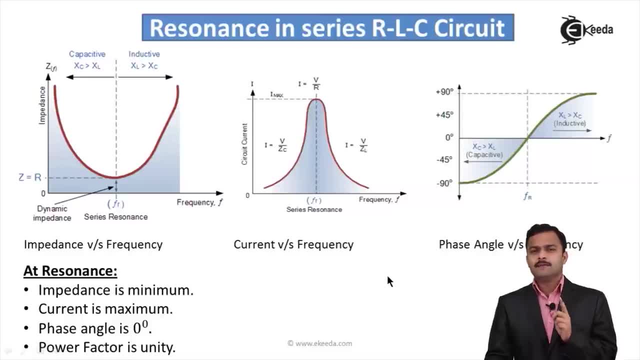 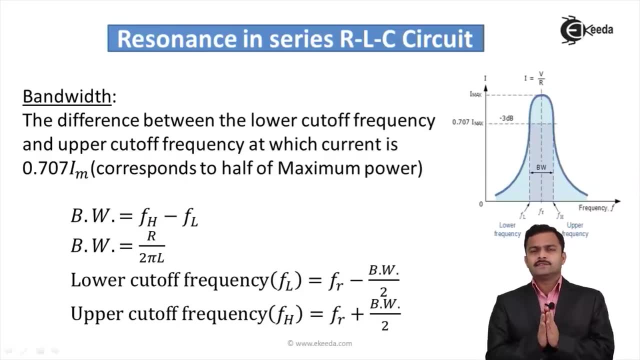 resonance and power factor is unity, which is maximum at resonance. Now we have seen a resonance once current, we come to know current is maximum at resonance. obviously, power is also maximum at resonance 10.1.. So what is the maximum at resonance? Is it minimum at resonance or less than zero? 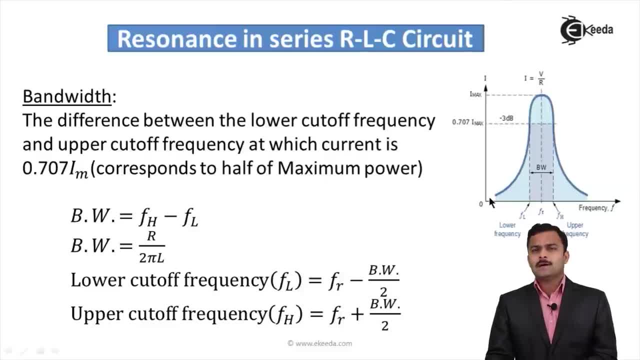 10.1.. So what is the maximum at resonance? Is it minimum at resonance or less than zero? here we are going to use the graph of current versus frequency to determine the most important parameter of a circuit, and that is called as a bandwidth. Bandwidth is nothing but a selectivity. 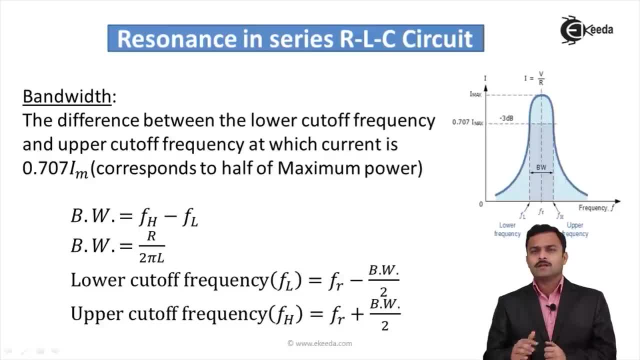 of a circuit to receive or give out the signal. So bandwidth is nothing but a frequency range in which signal is accepted, and those frequencies which are called as a lower cutoff and upper cutoff are nothing but frequencies at which I am getting half of the maximum power, which 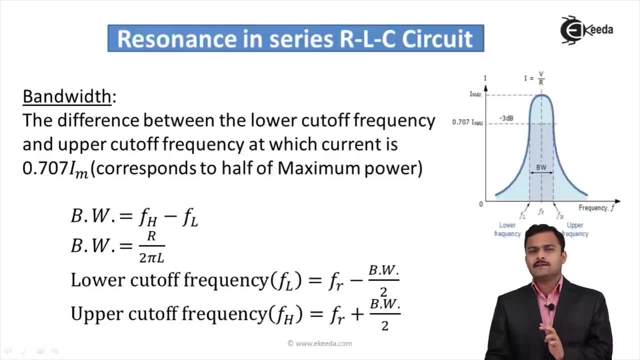 is correspond to 0.707 times the maximum current. So if I denote those values of the frequencies I will get here: lower cutoff frequency FL. upper cutoff frequency, FH. and the difference between them is called as a bandwidth. So the bandwidth is nothing but the difference. 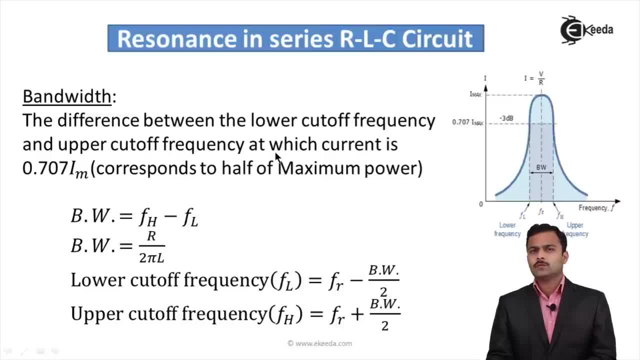 between the lower cutoff frequency and upper cutoff frequency. So the bandwidth is nothing but the frequency at which current is 0.707 IM. IM is the maximum current and that is corresponding to maximum power. So bandwidth formula is FH minus FL. In terms of parameters, 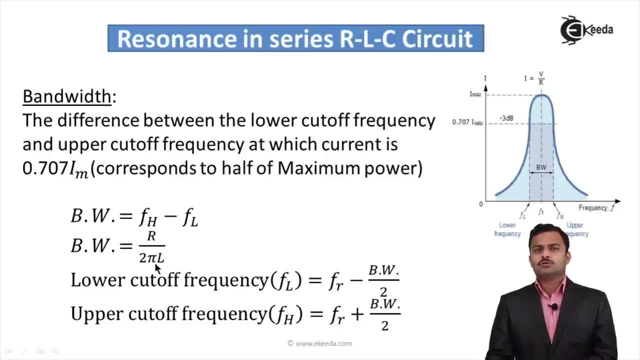 of circuit. bandwidth is given by R upon 2 pi L. So if I know the value of resistance of circuit, if I know the bandwidth, I can get a lower cutoff frequency. So lower cutoff frequency, FL, is nothing but FR minus half of the bandwidth. Same way upper cutoff frequency. 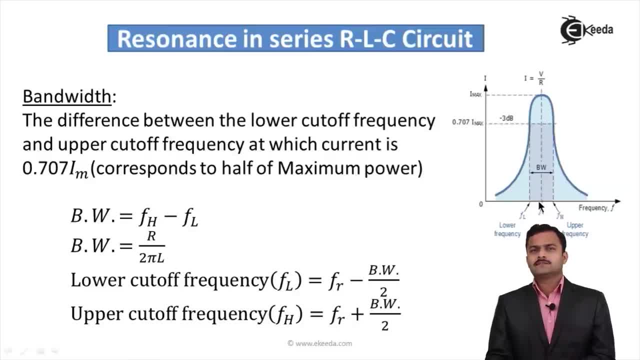 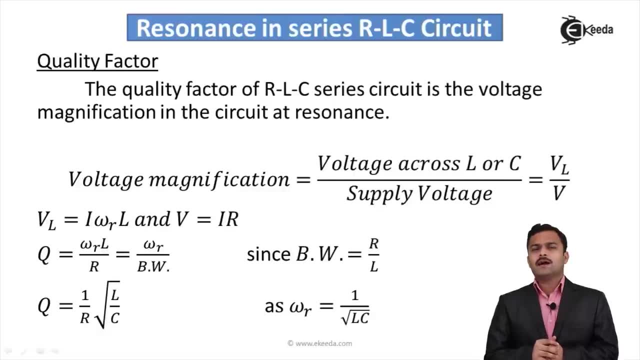 I can say FH equal to FR plus half of the bandwidth. Now one more important part for a series- resonance is a quality factor. So the quality factor of a series RLC circuit is the voltage magnification in the circuit at resonance. I will explain. 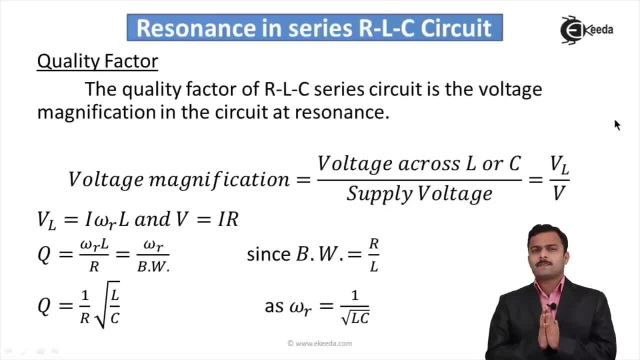 voltage magnification. Voltage magnification is nothing but voltage across L or C divided by supply voltage. It may happen that you are supplying a voltage of 10 volt to a series RLC circuit, But voltage across inductor and voltage across capacitor you may get 100. 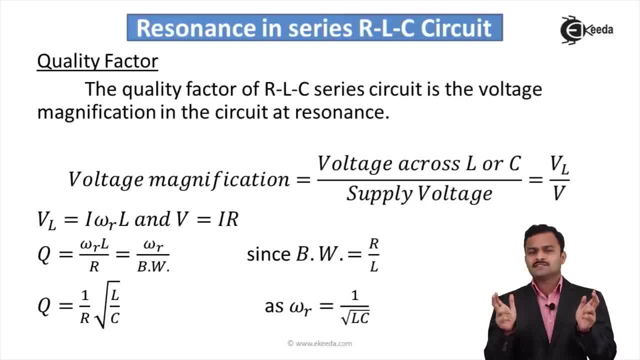 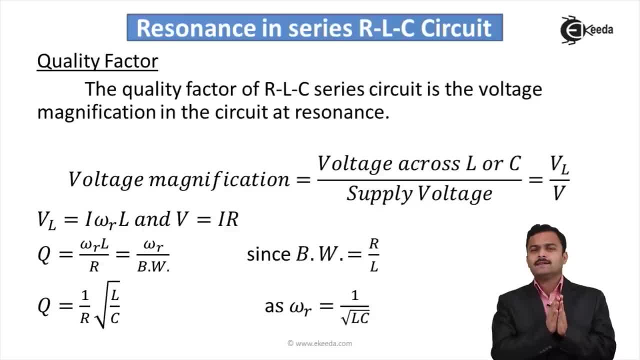 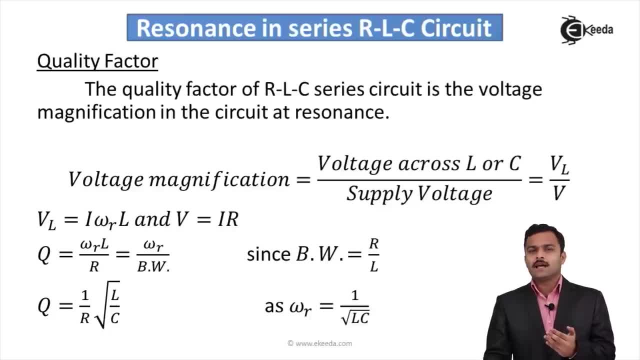 upon what is the value of L and C and, obviously, resonating frequency. So what happened? 10 volt is getting magnified upto higher voltage level because of resonance phenomena. Therefore it is called as a voltage magnification, also called as quality factor of series resonance. 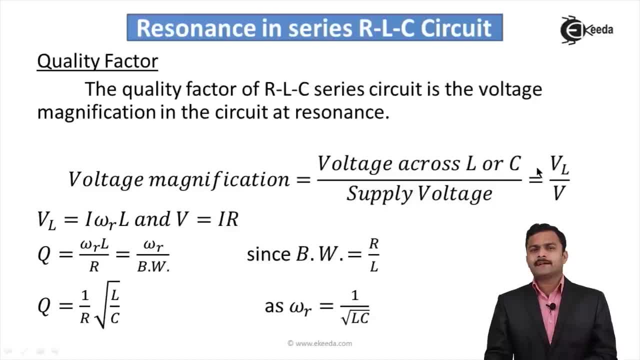 So VL or VC at resonance is nothing but I into XL or XC at resonance, and XL is given by omega RL and supply voltage. everybody knows supply voltage is nothing but a voltage across resistance only, which is I into R. So if I substitute I will get Q equal to omega RL. 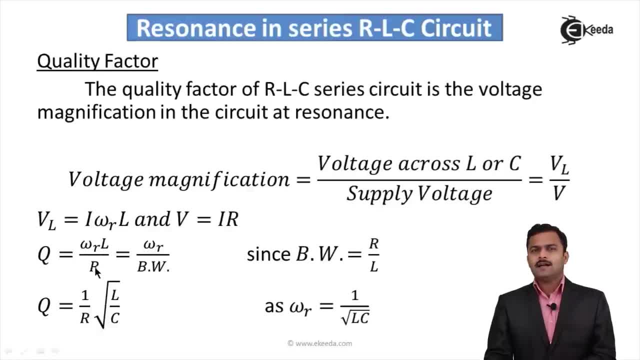 divided by R and R by L is nothing but a bandwidth. So it is one more formula for a quality factor which is omega R divided by bandwidth. omega R I will consider as 1 upon root of LC. So if I substitute 1 upon root of LC over here, what I will get? quality factor as 1 by R root. 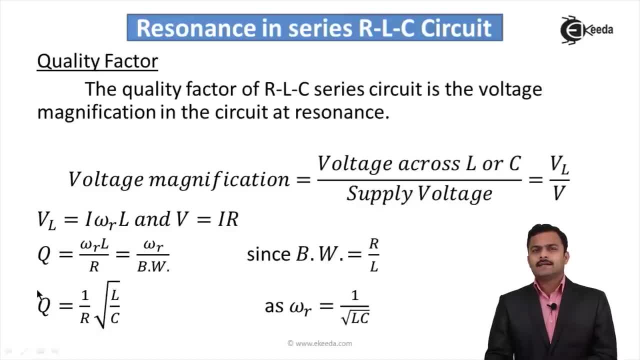 of L by C. So here I get a quality factor in terms of all the three passive elements. meaning if I know value of RLC, I can say what is the quality factor of the circuit? Quality factor is nothing but that factor which will get. 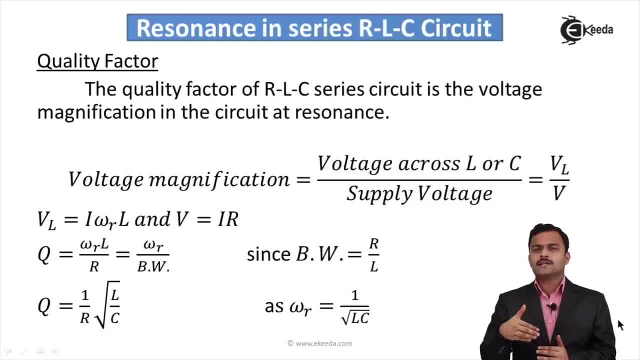 multiplied to the supply voltage in order to get a voltage magnified value. Series RLC circuit at resonance is also called as acceptor circuit. Why? because at resonance current is maximum, So I can say. So I can say current is getting accepted at a higher level at resonance. therefore series RLC circuit.